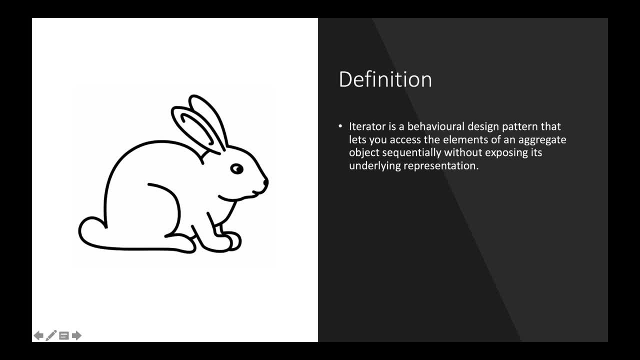 representation. So the intent of this design pattern, as you can see here, is that it lets you representation. let's take a look at the UML diagram and try to understand. how does iterator fit into this? the UML diagram: as you can see, a client has. 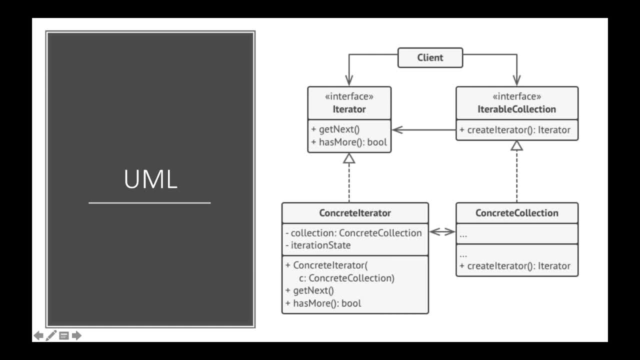 access to two different interfaces. the first interface is iterator and the second interface is iterable collection- both you can see that this iterator has a get next and has more method, which returns a boolean. so what this iterator will be doing is this will be having a reference to a collection. it we are. 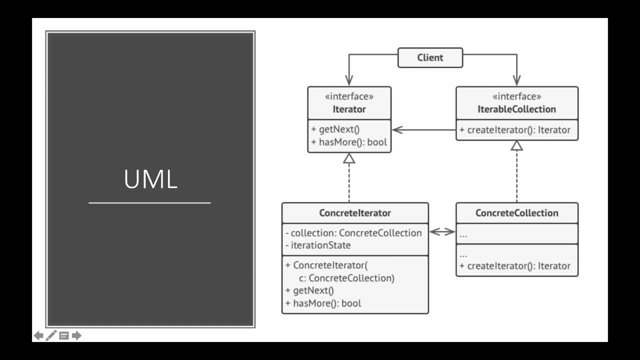 trying to iterate on, and it will have the functionality to, or it will have the logic to, get the next member from that concrete- I concrete collection and similarly this has more method- will be checking whether the collection has more values or not. so basically it's it's like until the collection has more. 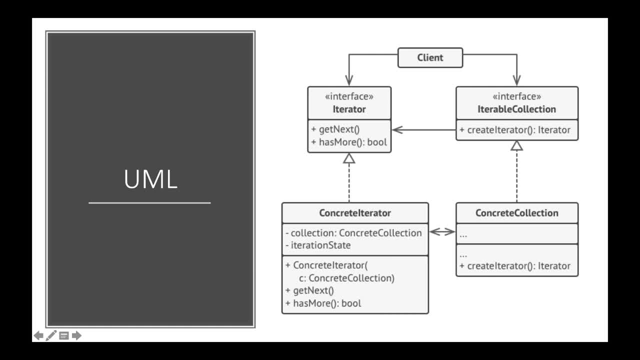 values. you can actually get the values from the collection. there is one more abstraction introduced here, which is the iterable collection. so the iterable collection has a method called a create iterator, and every collection which implements this iterable collection has to provide the implementation for the create iterator method. and what this client will do is it. 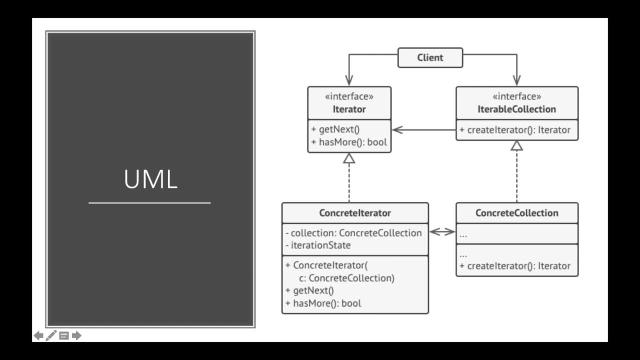 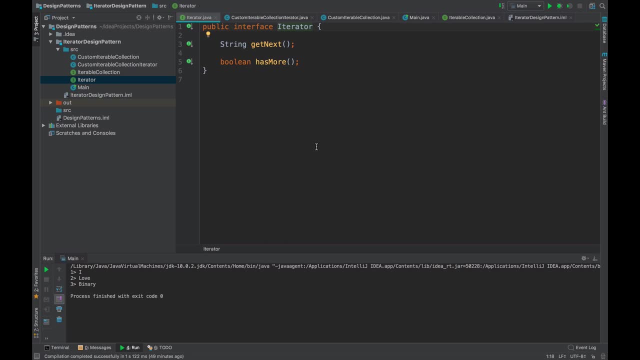 will use this iterator and the iterable collection interface to actually carry out or to actually access the object underneath. so this is a rahmancomus. so this is the coding example I was talking about, and I have created a one-to-one mapping from the UML diagram into the code, so it's very easy for you. 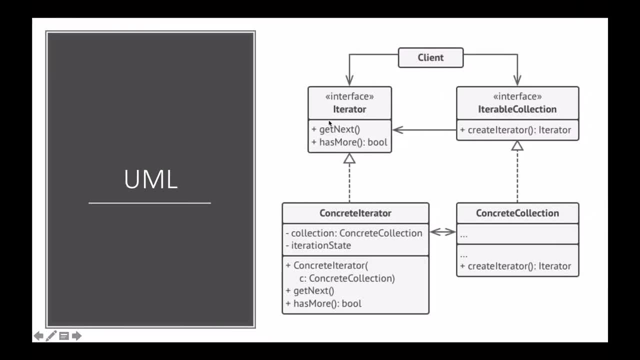 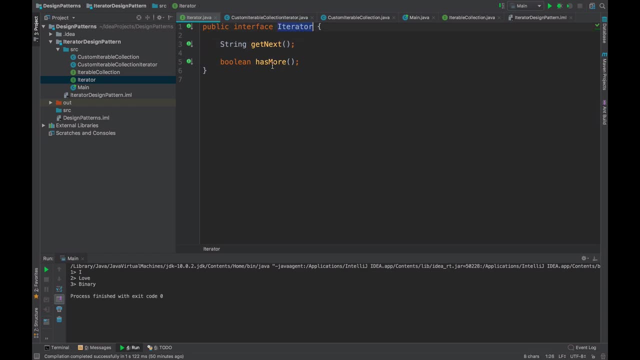 guys to understand it. the first interface which we saw in the UML diagram was the iterator interface which has a get next method and a has more method which returns a boolean. similarly, we have also defined a get X method in interface, called iterator, and it also has a method which returns a boolean. 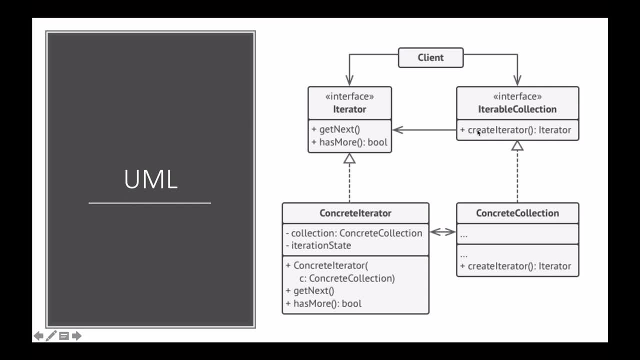 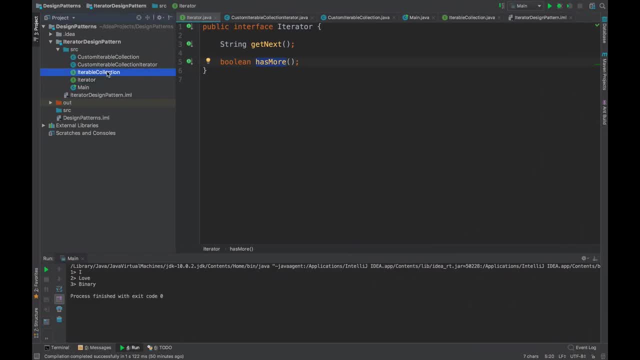 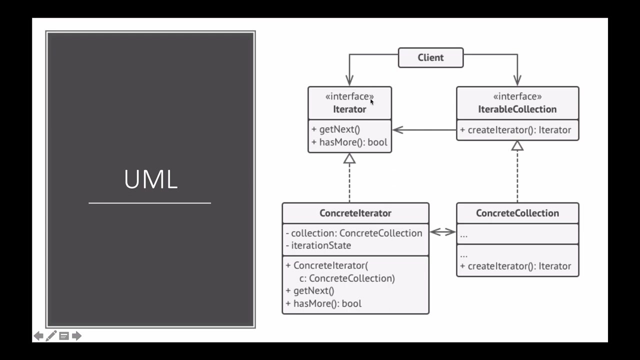 next, we have a iterable collection interface which has a create iterator method, which returns an iterator. so let's go to our iterable collection interface, which has only one method, which is called the create iterator method, which returns a iterator. apart from these, we have two more classes: which is a concrete iterator, which implements. 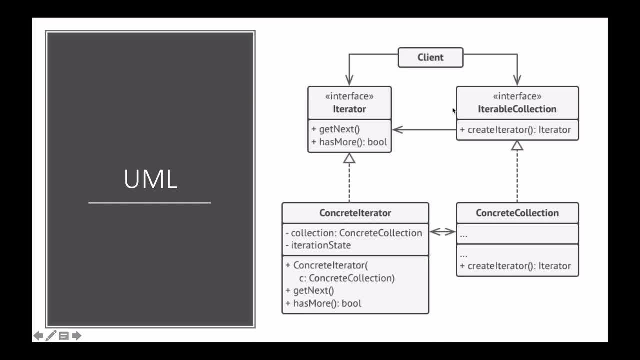 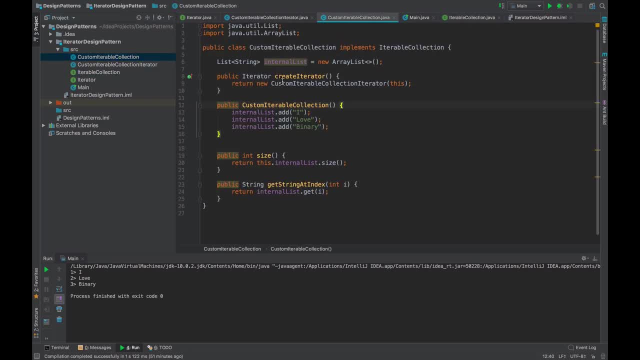 iterator and we have a concrete collection which iterates iterable collection. so we'll first go and take a look at this concrete collection. so in my case, i have written this concrete collection to be composing a simple list of string which is- i have named it like internal. 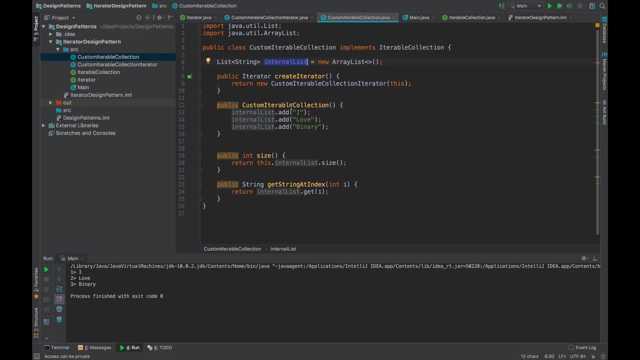 list and what i am doing is in the constructor of this custom iterable collection. i am going to be doing is that i am adding a string to the collection. i am adding- i love binary strings to this internal list. i've also added a size method for the convenience, so that i can know. 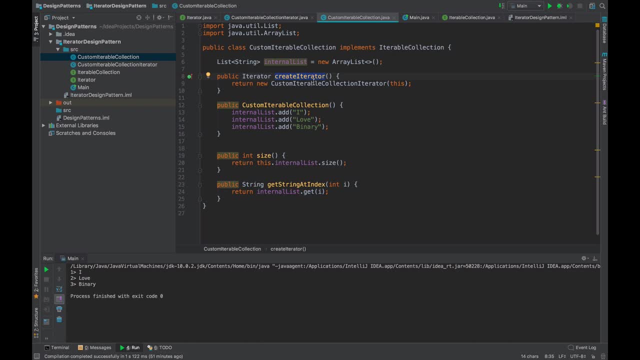 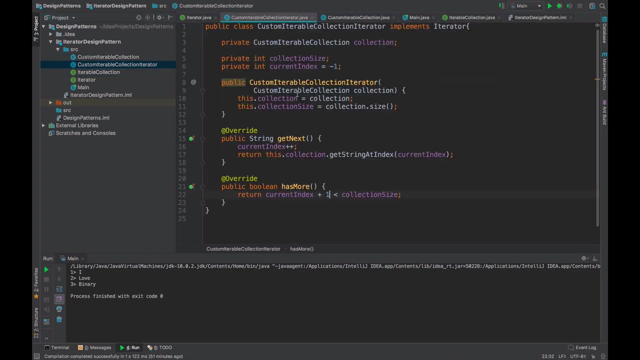 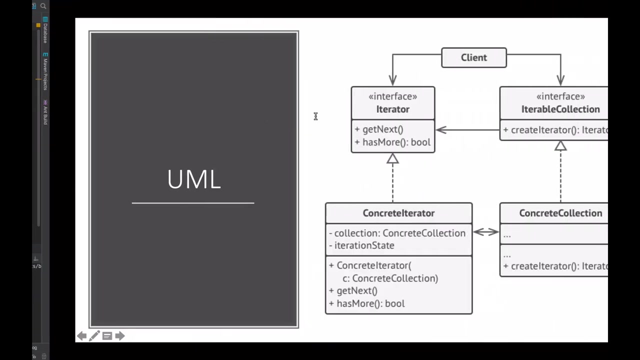 the size of my internal list and also i have written a create iterator implementation which will actually return a iterator instance which can be used to iterate over this collection, and that iterator instance is the concrete iterator defined as custom iterable collection iterator, which implements the iterator and, as you can see, this has a reference to a concrete collection, since we have a concrete. 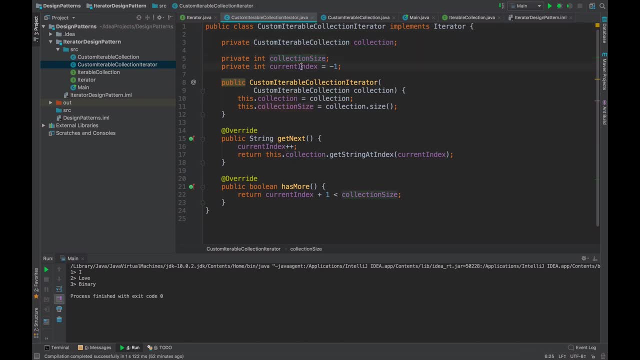 collection reference and this maintains some collection size and current index of the collection. so in the constructor of this iterator, which is called via the collection, we initialize this internal collection reference as the collection which called or created this iterator. at the same time, we also set the size for the collection and we have implemented the 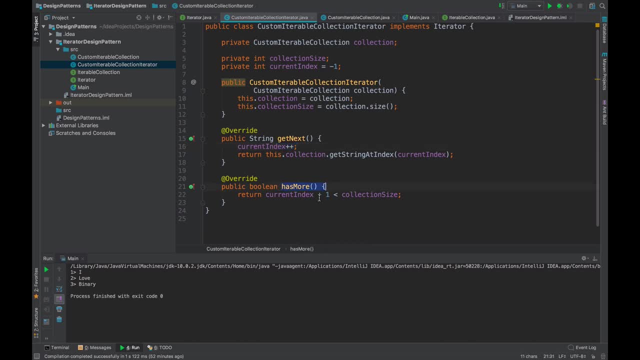 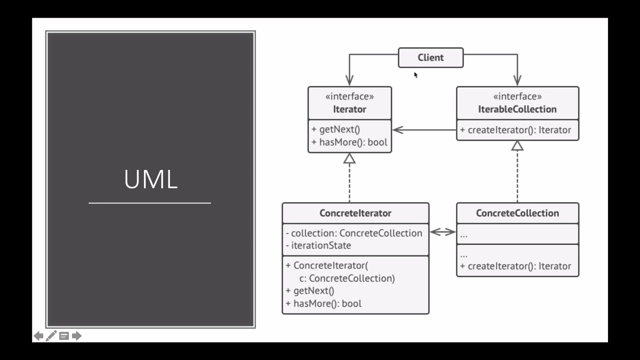 get next method and we has more method to actually check for any more instances in this collection and if there is, we will return it via the get next method. so the main part of this program is this client method, which will use this iterator and iterable collection interface. 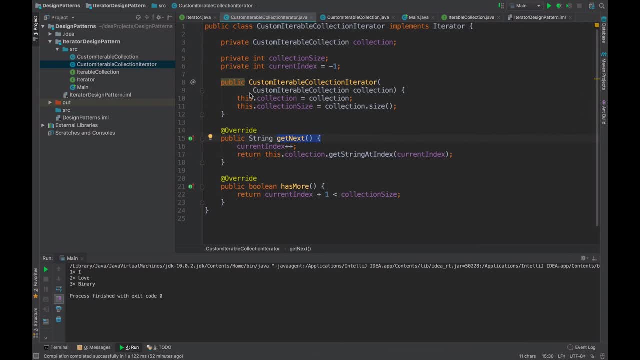 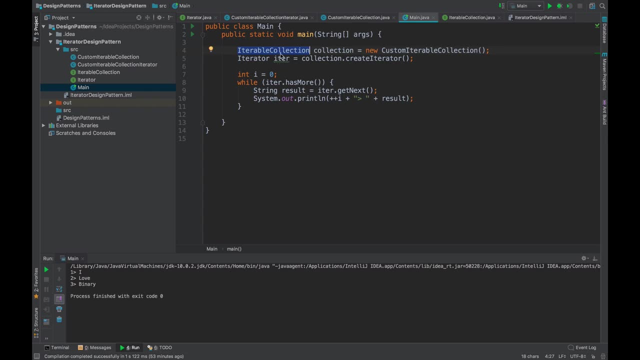 to actually iterate over the collection and get the values. so this is actually that client method. as you can see, it has iterable collection, which is an interface, and it also has iterator, which is an iterator for this collection, and this client method is using this iterator. dot has more method.